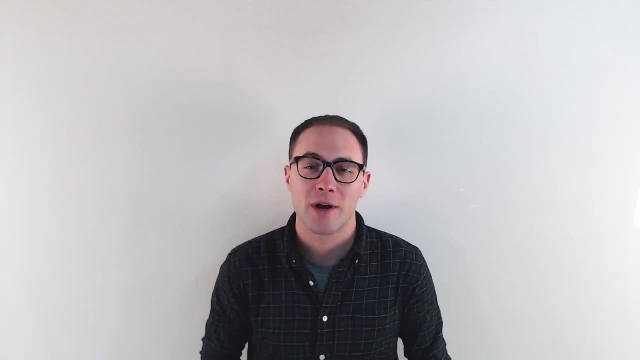 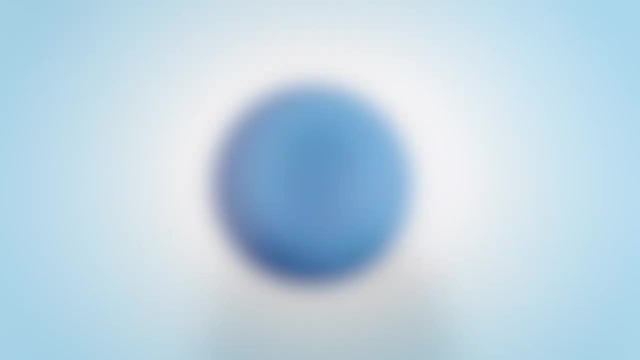 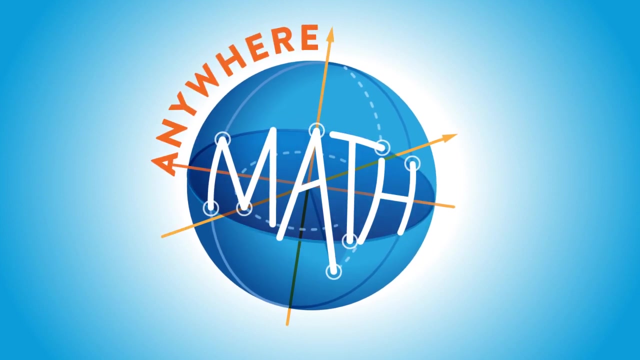 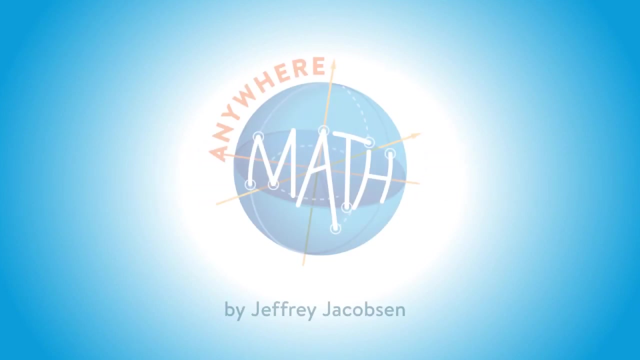 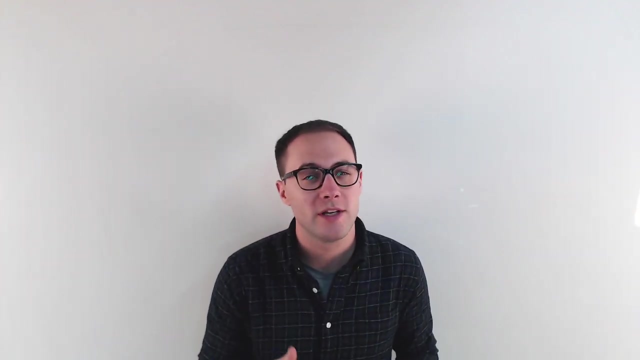 Welcome to Anywhere Math. I'm Jeff Jacobson and today we're going to be comparing and ordering fractions, decimals and percents. Let's get started. Before we get to the first example, there's one main rule you need to know when you're comparing or ordering fractions, decimals and percents. 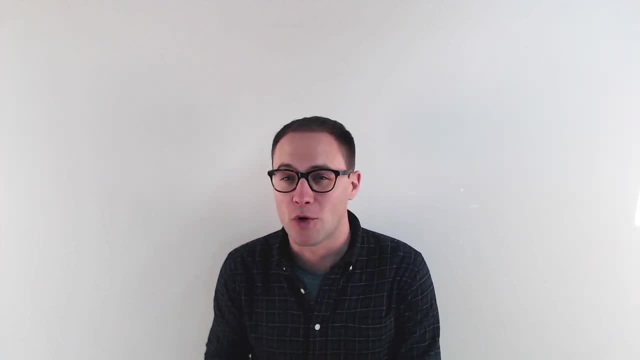 You may have heard the phrase: it's like comparing apples and oranges. That's a very common phrase and basically what it means is: it's hard to compare apples to oranges. They're different, right. Same thing with fractions, decimals and percents. 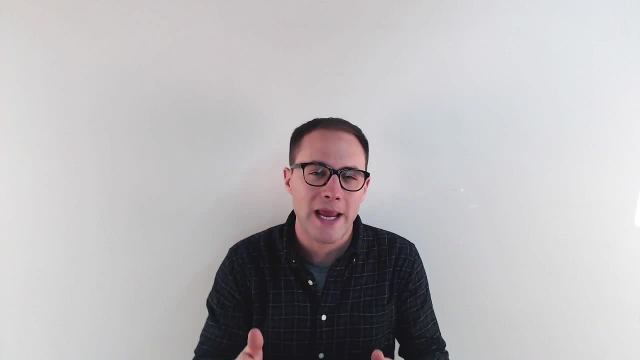 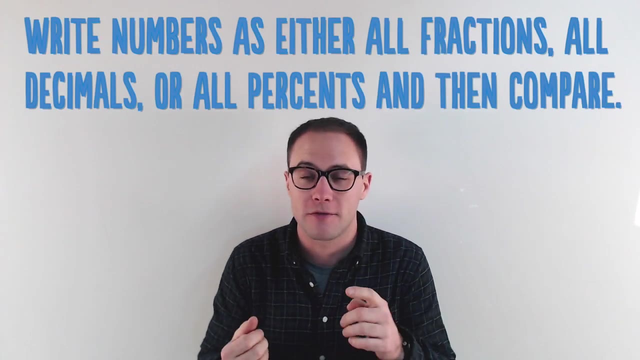 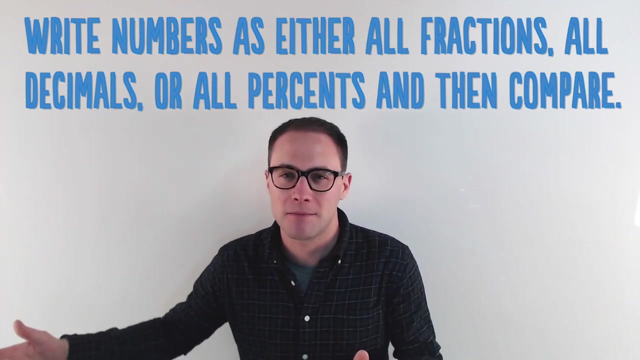 We can't compare them when they're all different. So the main rule with comparing and ordering fractions, decimals and percents is that you have to make them all- either fractions, all decimals or all percents- and then compare them. If they're not all the same, you can't compare them. 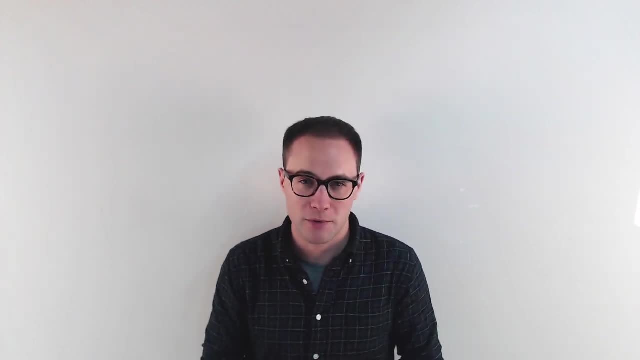 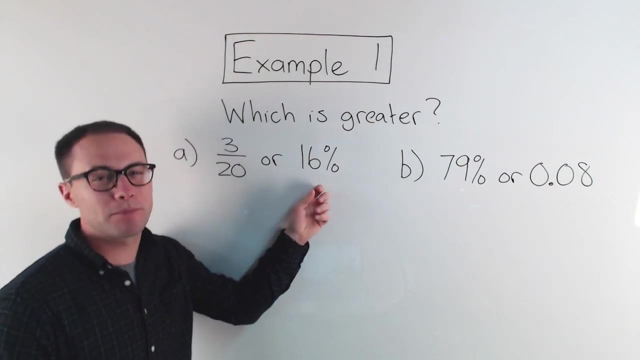 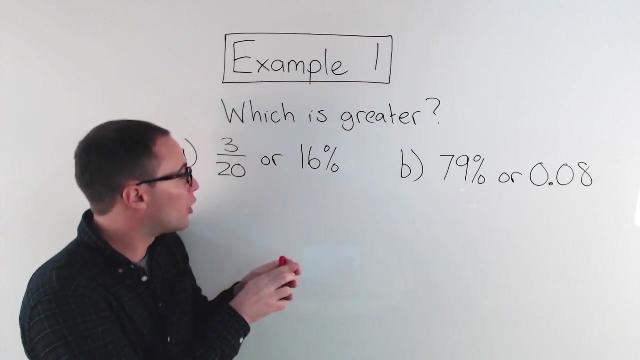 Okay. So with that in mind, let's get to our first example, Example, one which is greater. So we're comparing: here we've got three twentieths compared to sixteen percent. We're comparing a fraction with a percent. Now, again, the main rule you've got to make them, in this case, both, either fractions or both percents. 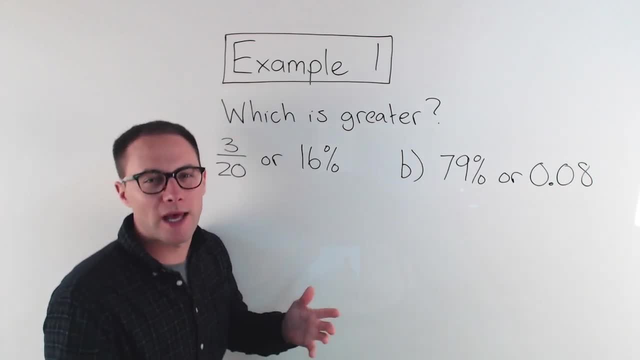 Most of the time, either one will be okay. There's one main thing that you should keep in mind, though: when you're comparing, When you're comparing or ordering, and you're having to change things into fractions, decimals or percents- decimals and percents are fine. 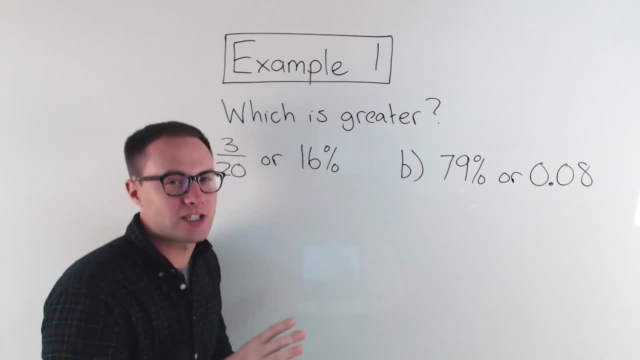 Right, They're no big deal. If you change everything to fractions, then sometimes you're going to have an extra step, Because in order to compare fractions you also need common denominators. So when you do that, sometimes you're going to have extra work to be able to do that. 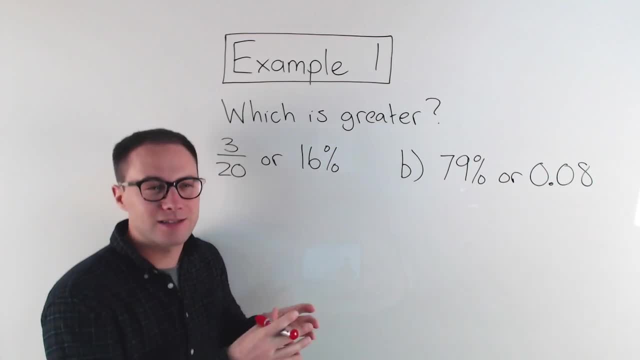 So oftentimes making them all into fractions, that's not going to work. fractions is usually maybe not the best choice, so keep that in mind when you're doing these problems. so here we go. part a: 320 is, or 16%, so do we want to make? 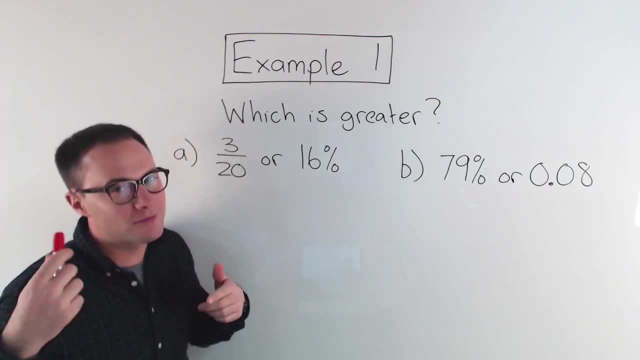 them both fractions? or do you want to make them both percents? and if you remember what I just said, in my opinion I think it's going to be easier to make them both percents. well, 3 over 20, remember, percent means per 100, so it'd. 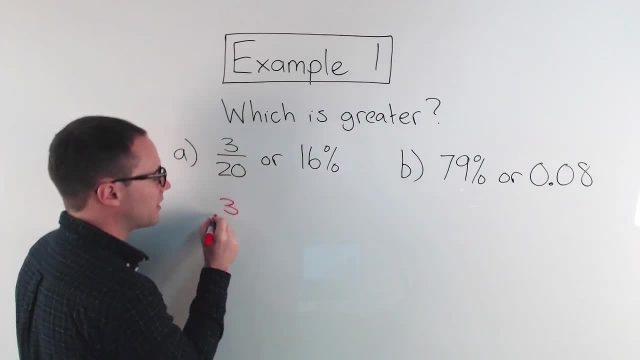 be great if this denominator was 100. well, that's easy for us to do 3 over 20. if I want it to become over a hundred, well, to do that, all I need to do is multiply the denominator by 5 and if I do that to the denominator, to make an. 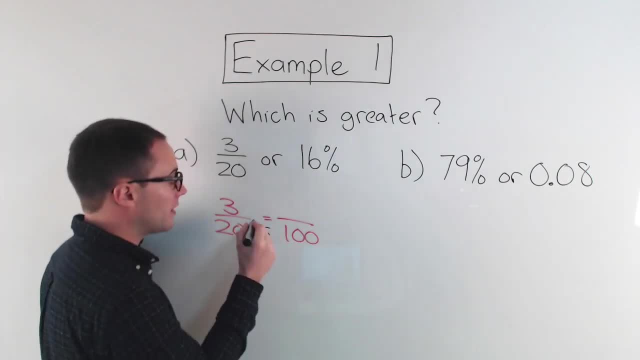 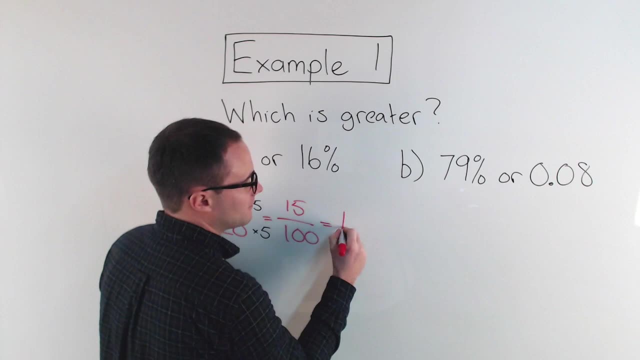 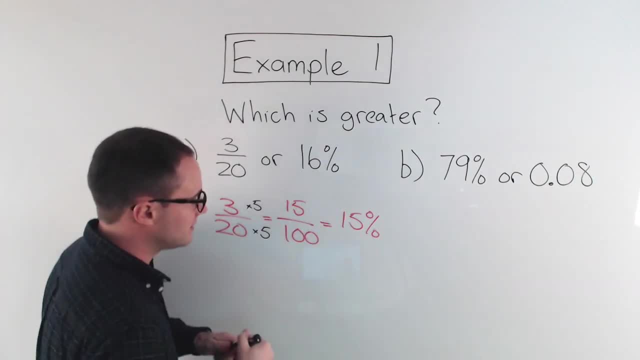 is the same as 15% or 16%. well, that's easy. 16% is greater than 15%, so it's greater than 3- 20th. so see how easy it becomes once when they're both the same, both percents, then it's really easy to compare. 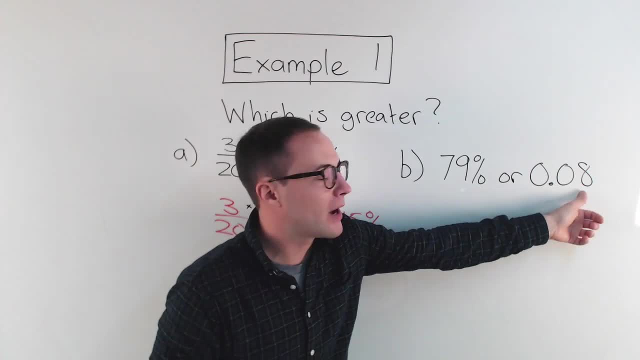 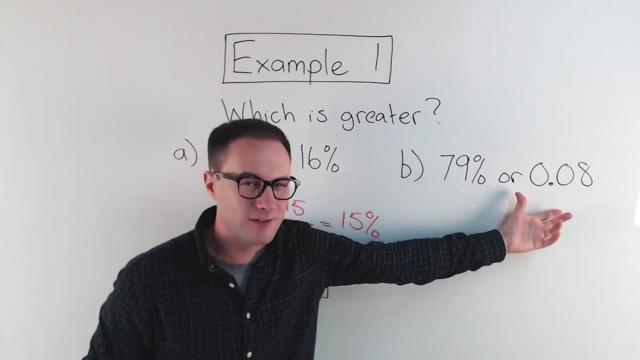 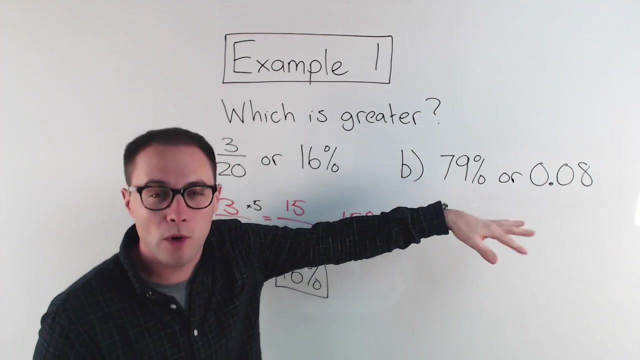 let's try B, 79% or 0.08. so in this case we've got two options, and either would be fine. I can make both of these percents fairly easy, easily, and I could also make them both decimals quite easily. so either one works, you don't. 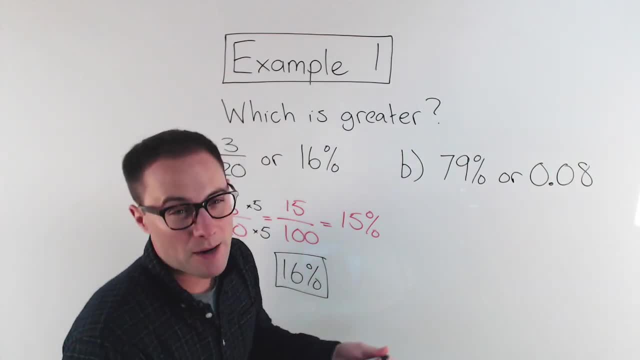 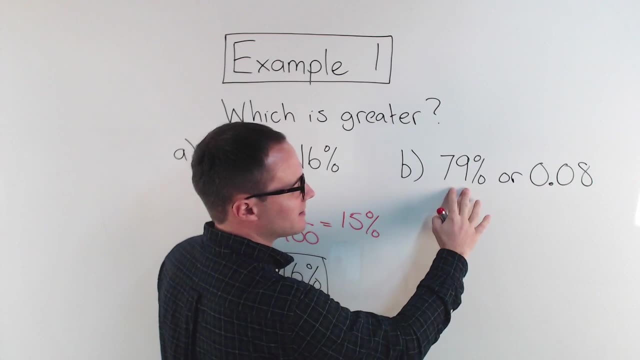 have to worry about fractions. so let's see how about we do both. if I'm going to compare them both as decimals, well then I would need to make this as a decimal, and percents to decimals is easy. I just moved the decimal place twice to the. 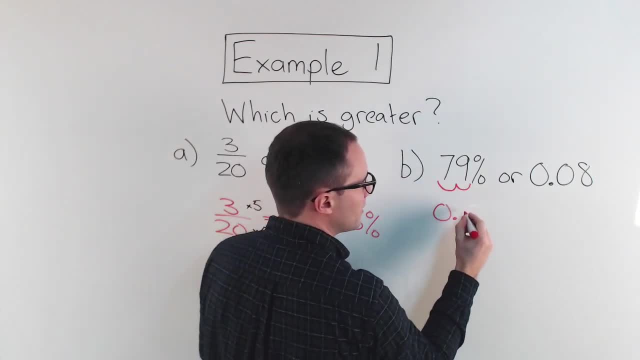 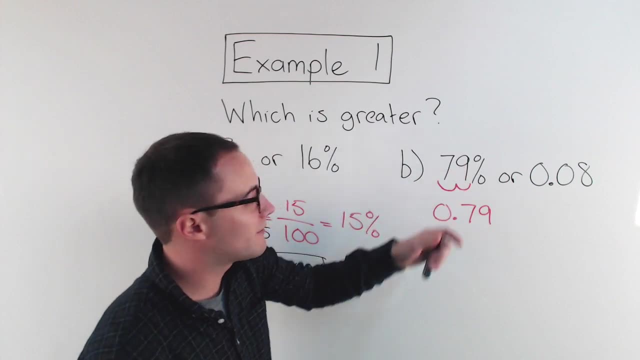 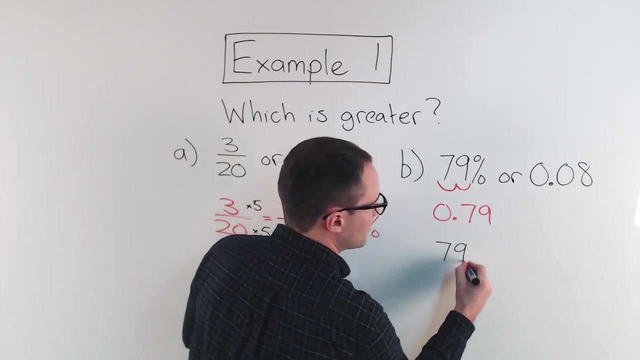 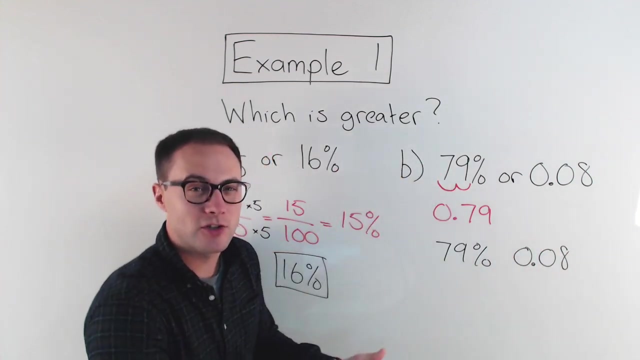 left one, two, which would mean 0.79. okay, well, 0.79 is greater than 0.08, which means 79% is greater. let's try the other way. let's make this a percent, so again I'll have 79%, and I'm changing 0.08 to a percent, decimals to percent, you just go. 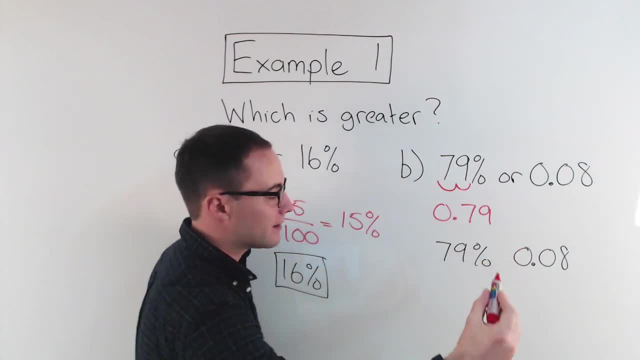 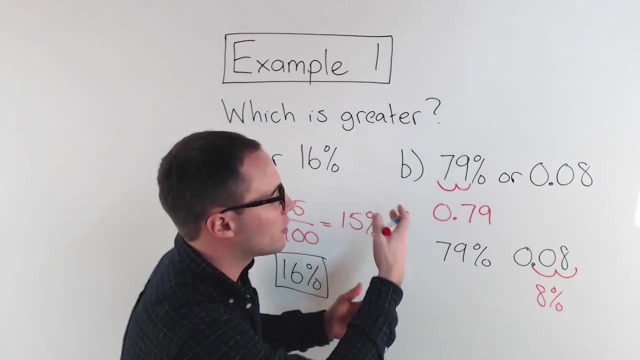 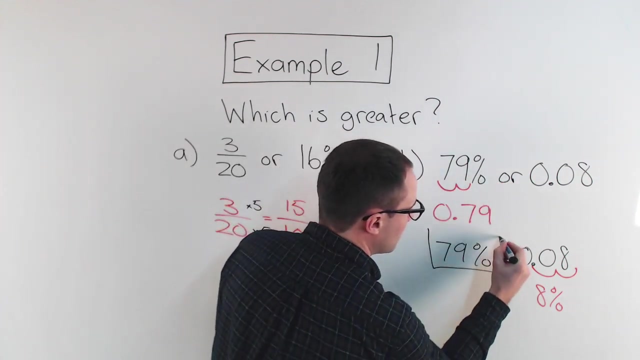 the other way. I move the decimal point twice to the right, so one, two and it becomes eight percent. so same thing. either way I do it, 79% is going to be greater than 0.08. so that is greater. okay, here's something to try on your own. 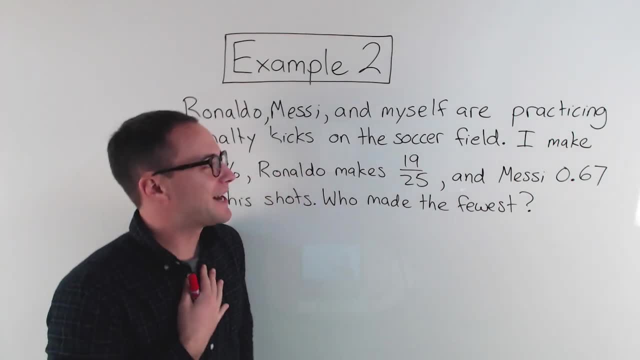 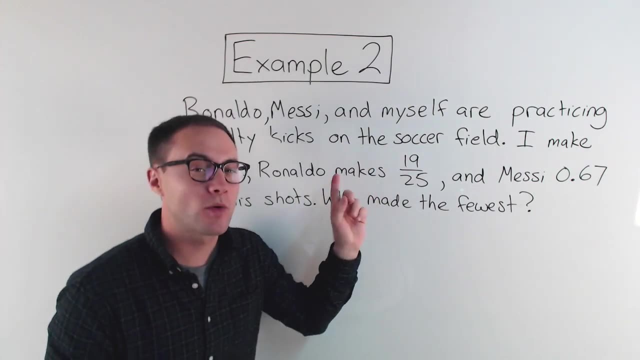 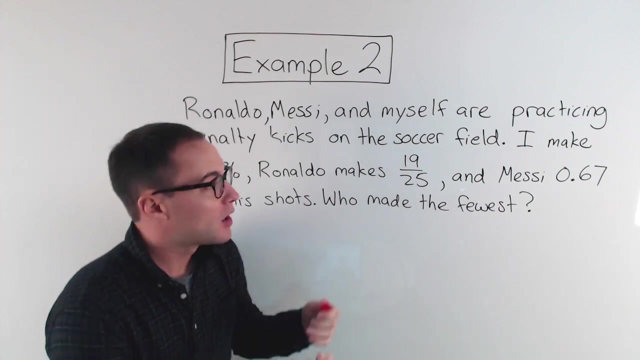 example two: Ronaldo, Messi and myself are practicing penalty kicks on the soccer field. I make 72 percent of my shots, Ronaldo makes 19 out of 25 of his and Messi 0.67 of his shots. who made the fewest? well, first let's underline our important 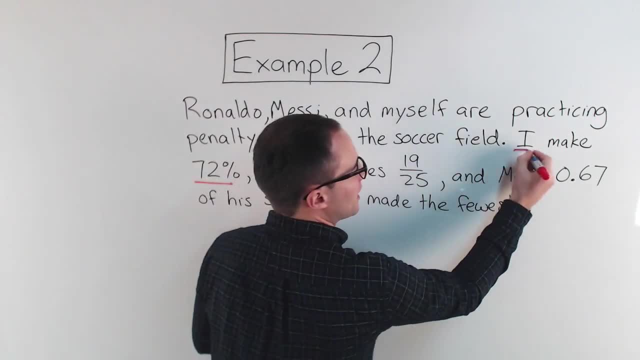 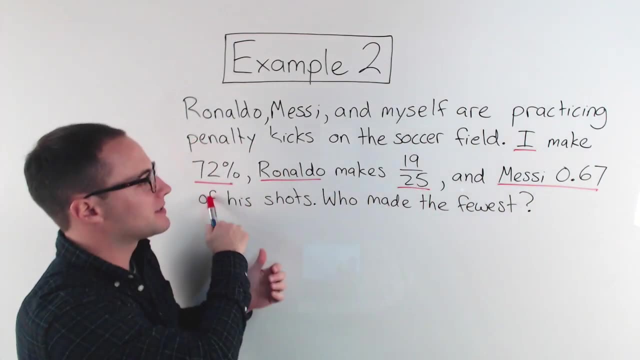 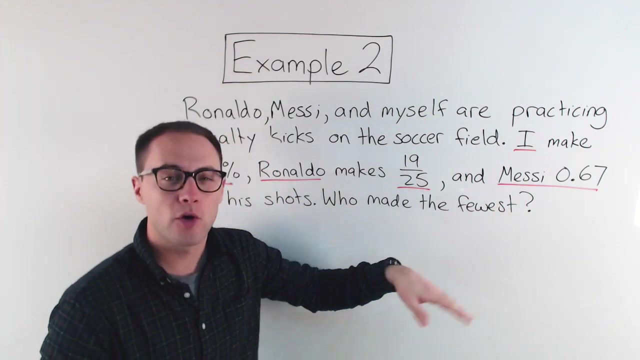 information. so I make 72 percent, Ronaldo 19 out of 25 and Messi 0.67. so notice, we've got a percent, a fraction and a decimal. okay, we're gonna have to compare all of all three of those to find out who made the fewest. now to kind of be a little happy, somewhat organized, I'm. 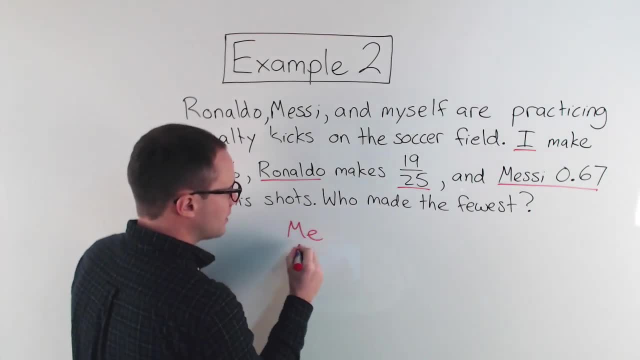 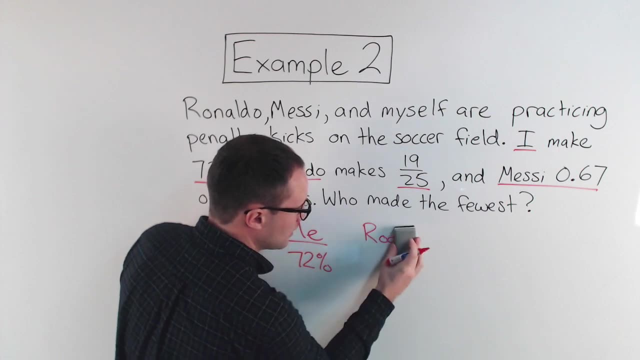 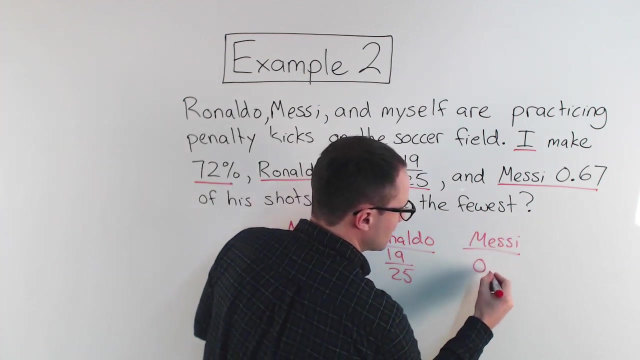 just gonna make a little bit of a table. so here's me with 72 percent, then we've got Ronaldo. whoops. and we've got Ronaldo, at what was he? 19 out of 25.. And then we've got Messi with 0.67.. Okay, Now, if you were going to use logic, you would. 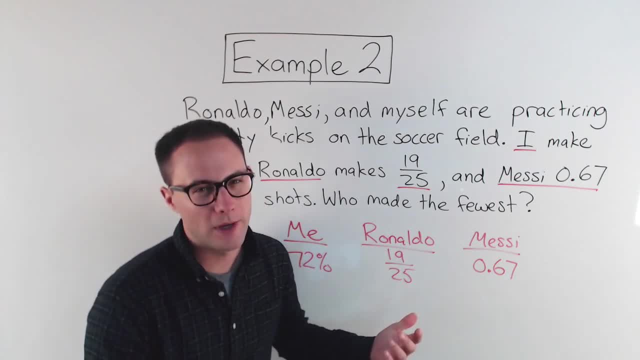 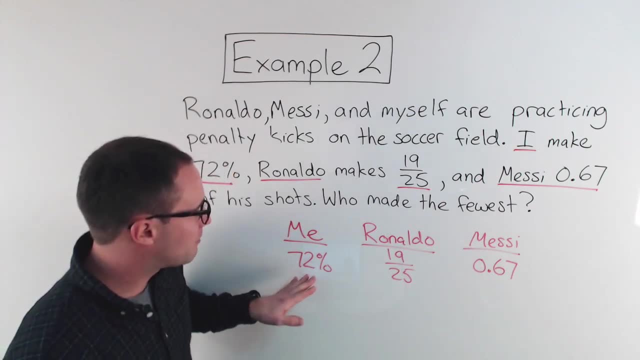 probably say: oh well, it was probably Ronaldo who made the fewest right. Obviously, it's not going to be me because I make all my penalty kicks, But anyways. so here we go. Percent fraction decimal- Again the rule we got. to make them all the same, We can make them all. 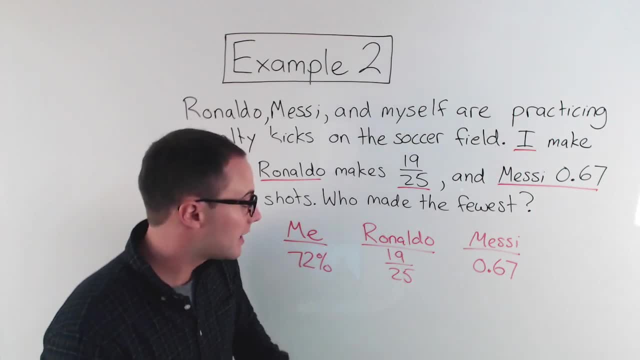 percents. we can make them all fractions or we can make them all decimals. Remember, fractions are going to be usually the toughest, So let's skip that And let's think: do we want to make them all percents or all decimals? And really it doesn't matter For me. I'm going to